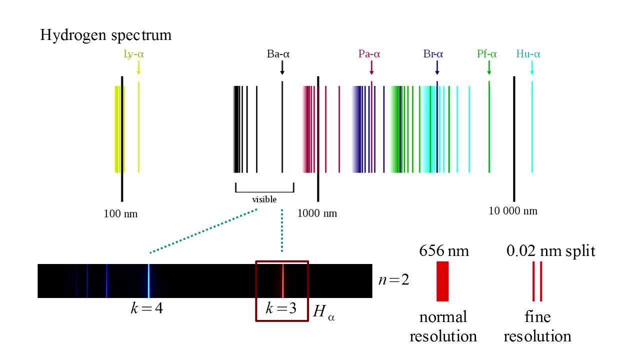 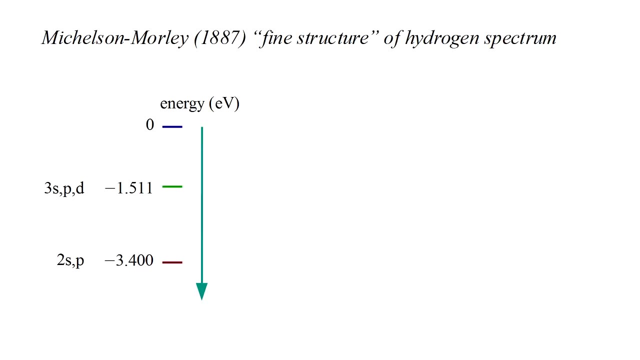 That's a split of only about 30 parts in a million. Further precise observations of other atomic spectra showed more examples of this. Here are more examples of this fine structure of spectral lines. With the development of the quantum theory of the hydrogen atom, it became clear that this implied a tiny splitting of hydrogen energy levels. 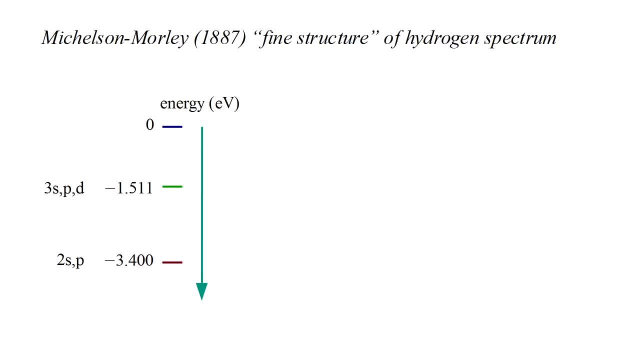 In video 6, we saw that the Schrodinger solution predicts that the different orbital types for a given energy level have exactly the same energy, But in fact precise measurement shows that the s-orbitals have single energy values, while the p- and d-orbitals are split into two closely spaced energy levels. 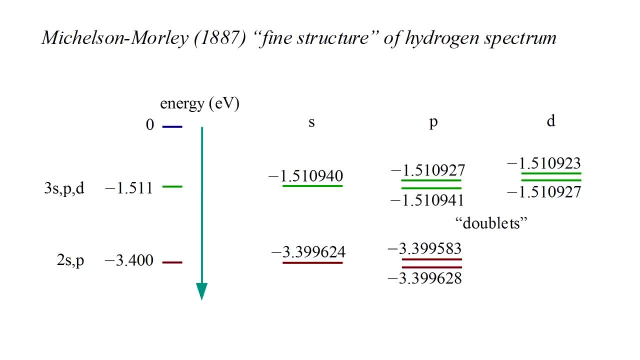 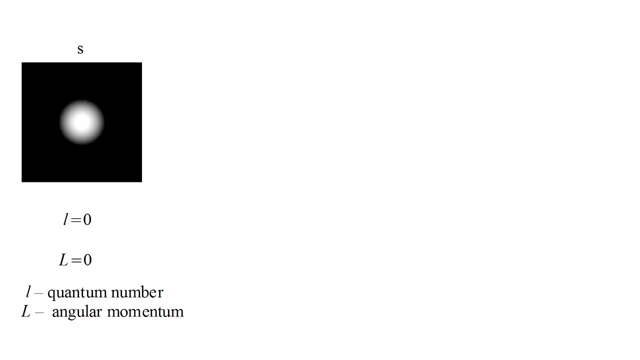 Y, single energies for the s-orbitals and double energies for the others. Recall from video 7,. s-orbitals have angular momentum number l equals 0. These are states of zero orbital angular momentum. In these states the electron does not, on average, go around the nucleus. The other orbitals have quantum number l equal to 1,, 2,, 3, and so on. In these orbitals the electron does have angular momentum. So apparently in orbitals with angular momentum the electron does not go around the nucleus. 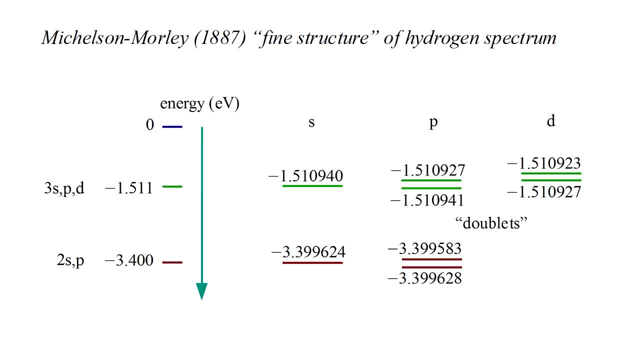 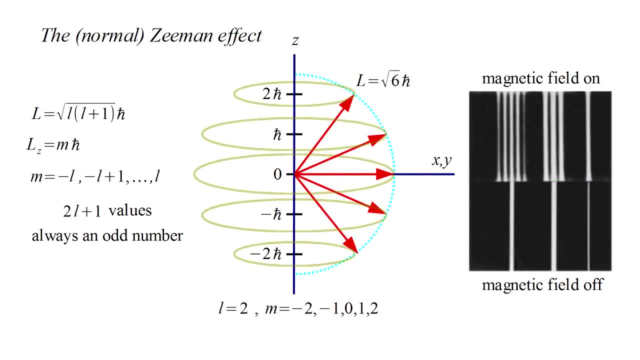 And so, basically, the electron does not go around the nucleus momentum. the energy level splits in two, but not in the s-orbitals, with no angular momentum. Why? Also, in video 7, we saw how an atom in a magnetic field can produce the Zeeman effect, where 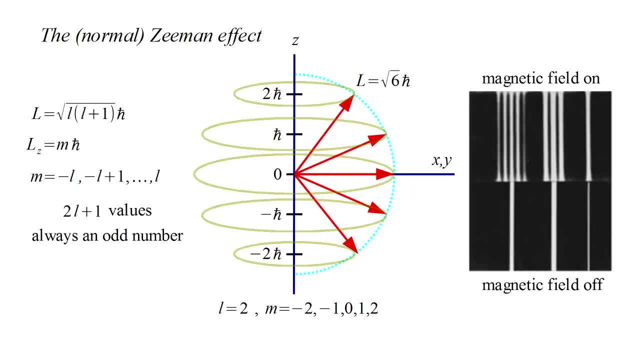 the electron orbital's energy changes for different z-components of angular momentum. Since there are always an odd number of possible components, the Zeeman effect shows up as a splitting into an odd number of lines, But in some cases the so-called anomalous. 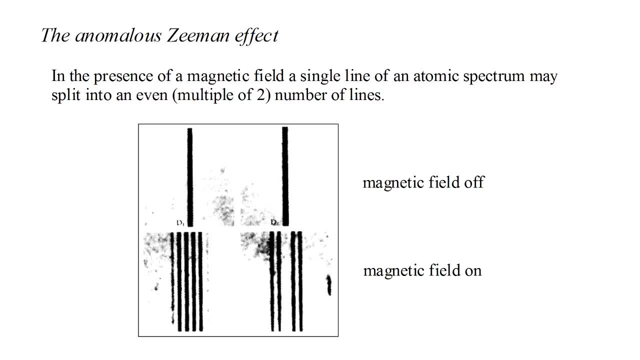 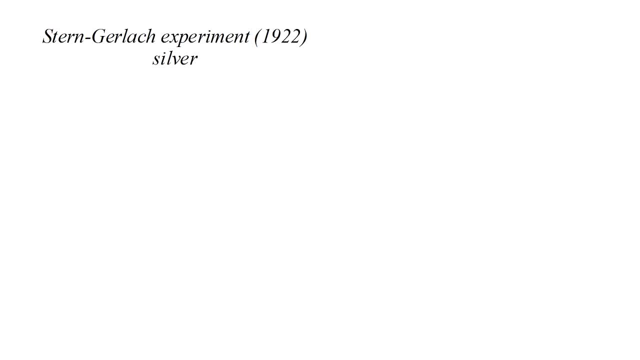 Zeeman effect, we see a splitting into an even number of lines, That is, a multiple of the number two. One of the most striking experiments characterized by the number 2 was the Stern-Gerlach experiment of 1922 using silver atoms. A similar experiment five years later by Phoipps and Taylor used 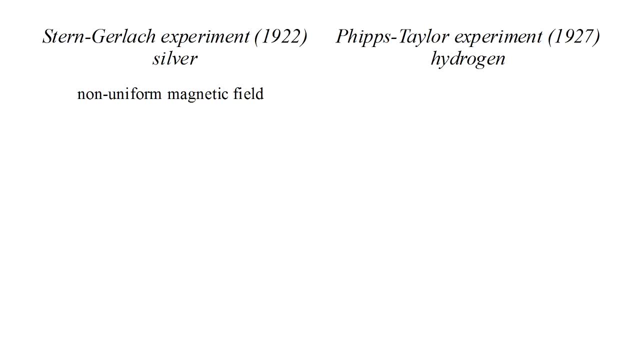 hydrogen atoms. These experiments employed a non-uniform magnetic field created by a magnet with different sized north and south poles. This causes the magnetic field to shift its weight to a new normal And that allows the magnetic field to rotate in a different way. This causes the magnetic field to change. 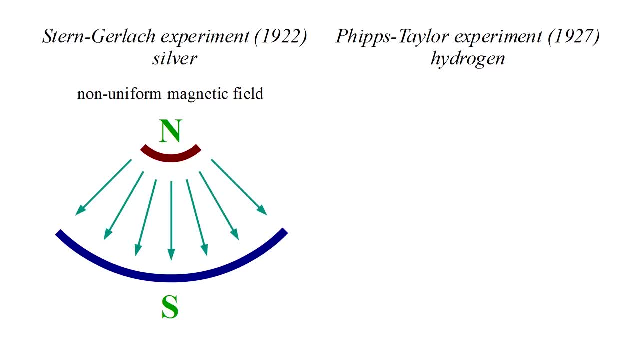 the direction of the wave. That causes the magnetic field to change. in this direction magnetic field is spread out, hence get weaker as we move from top to bottom. Suppose we now put a little magnetic dipole inside, with its south pole upward Opposite. 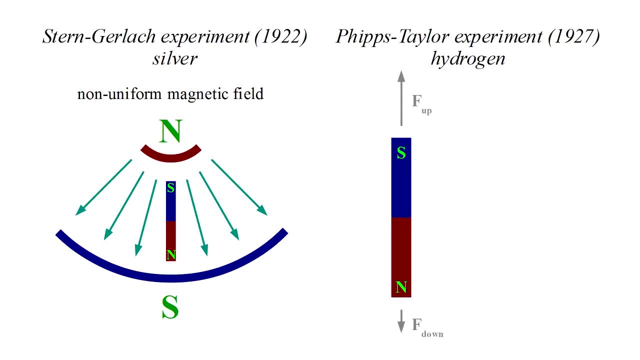 poles attract. so the dipole feels an upward force at its south pole and a downward force at its north pole. If the magnetic field was uniform, these would cancel and there'd be no net force on the dipole. But the magnetic field is stronger at the top, so the upward 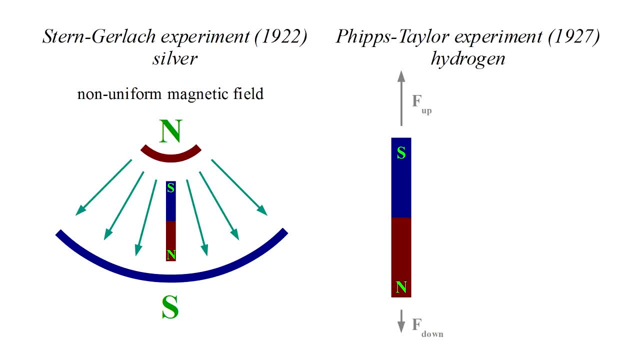 force is a little stronger than the downward force and there's a net upward force on the entire dipole. If we flip the dipole over, like poles repel, so the north pole feels a downward force and the south pole an upward force. Again, the top force is stronger due 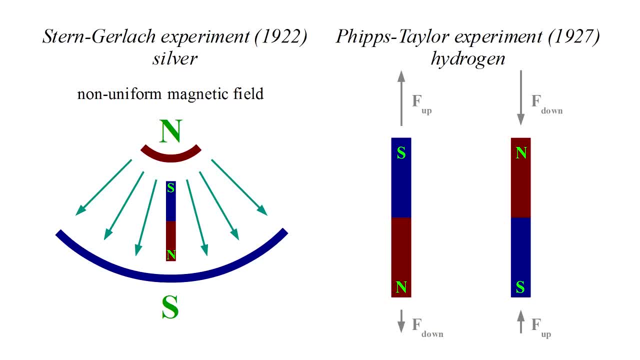 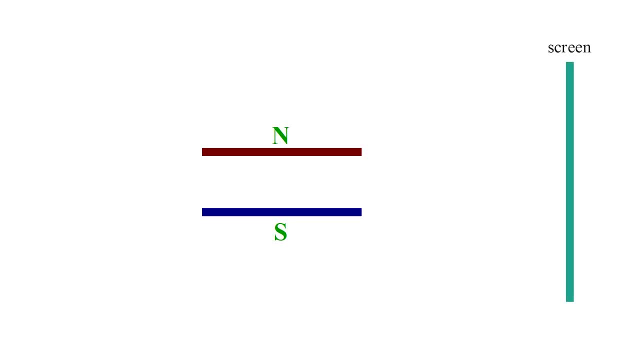 to the non-uniform magnetic field and the dipole feels a net downward force. Now consider a side view of our magnetic field. We put a screen at right and shoot uncharged atoms through the non-uniform magnetic field. If an atom has a magnetic dipole with its south pol up, the atom will curve upward. 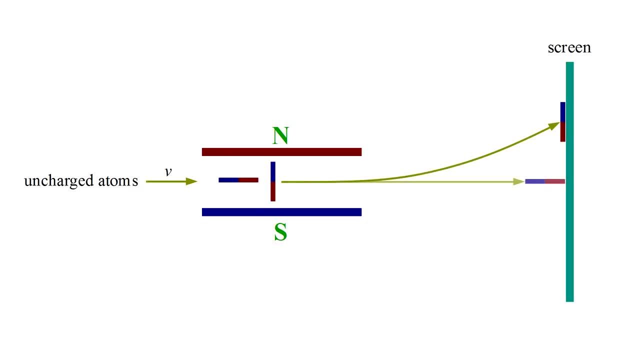 If the dipole is horizontal, there will be no net force and the atom will travel straight. If the dipole has its north pole upward, the atom will curve downward. Each dipole orientation will produce a spot on the screen. If these dipoles are due to orbital motion. 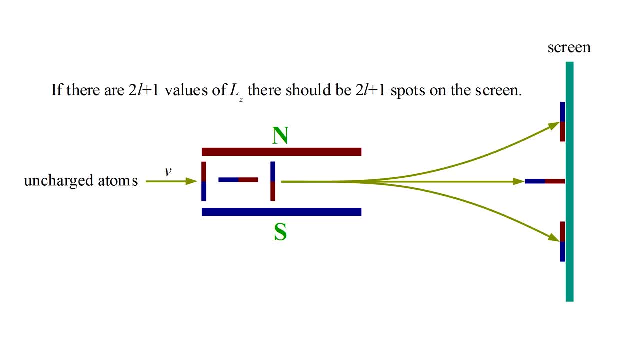 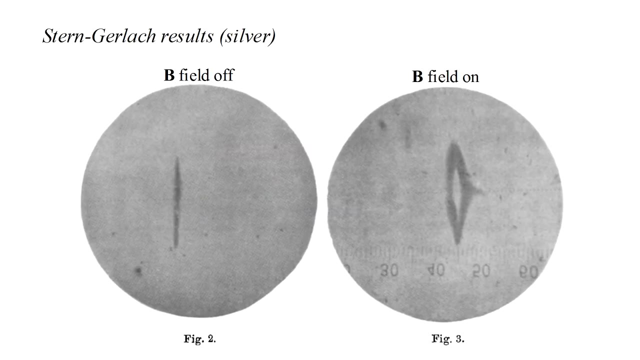 of an electron, then, as we've seen, there should be an odd number of spots. For silver and hydrogen, we should expect to see a single spot. However, both experiments found two spots. Here are Stern and Gerlach's results. for silver atoms, Their beam was more of a ribbon. 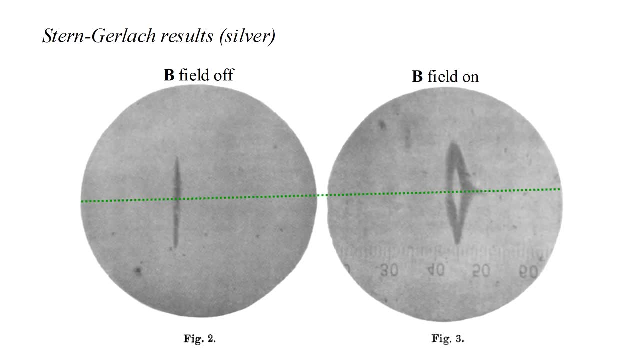 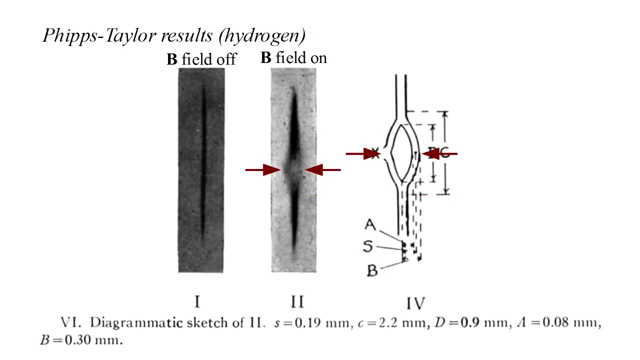 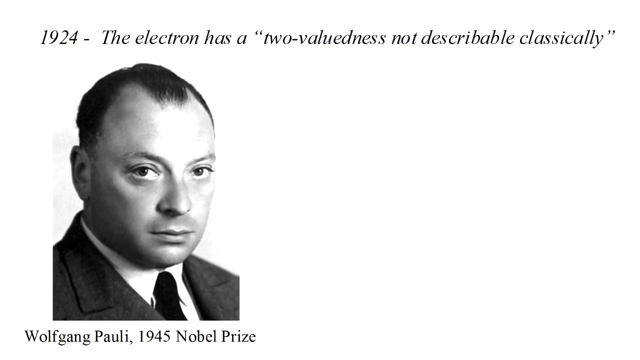 Along its center, where the magnetic field had the greatest non-uniformity, we clearly see the splitting in the two. Phipps and Taylor found similar results for hydrogen, although the experiment was more difficult and the effect was less pronounced. In 1924, Wolfgang Pauli proposed that these experimental results are evidence that the 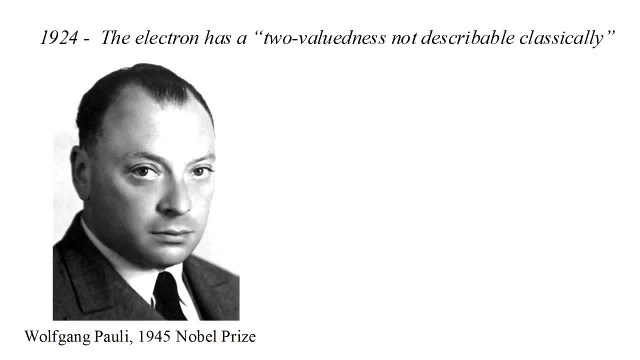 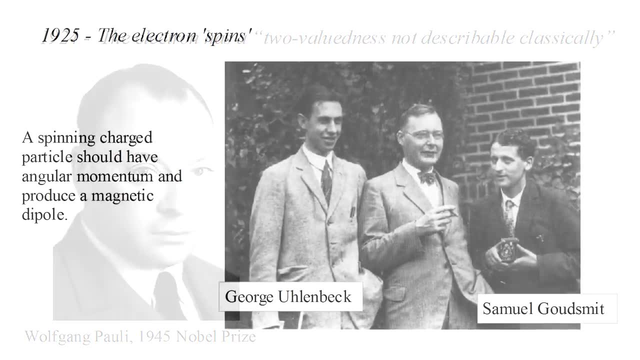 electron has a two-valuedness that is- quote- not describable classically. He was being very careful to avoid any analogy with classical phenomena. A year later, graduate students George Uhlenbeck and Samuel Gutschmidt proposed that the two-valuedness 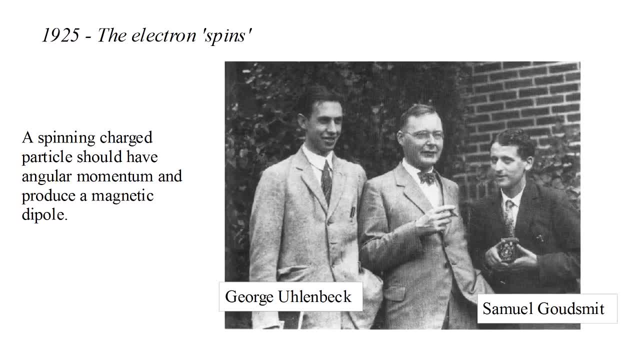 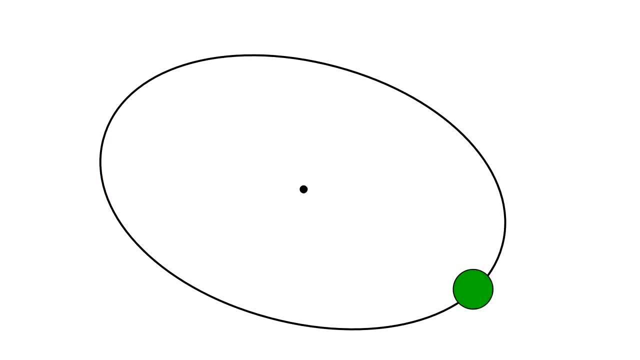 was due to the electron's spinning. Classically, a spinning charged particle should have angular momentum and produce a magnetic dipole. As we've already discussed, the motion of a particle around an orbit results in orbital angular momentum. If the particle is charged, as the electron is, this will also produce. 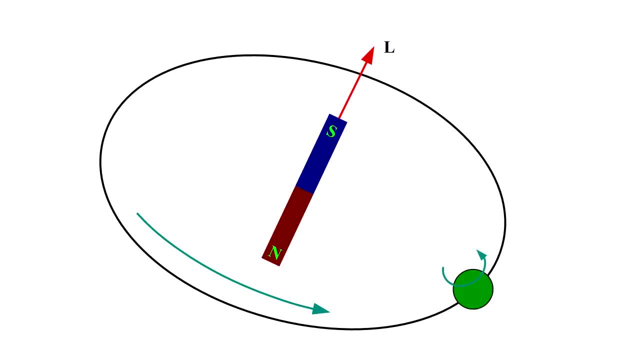 a small magnetic dipole. We might also envision the electron spinning about an axis analogous to the way a planet rotates. This would create another component of angular momentum that we'll label S for spin angular momentum, Since the electrons charged would also be spinning. the resulting electric current should also be spinning, as the magnet is spinning around an axis. If the electron was spinning, since the conductors charge the foot or the particle, the electrical would also be spinning. This would result in a spin. As we've already discussed, the motion of a particle around an orbit results in orbital. 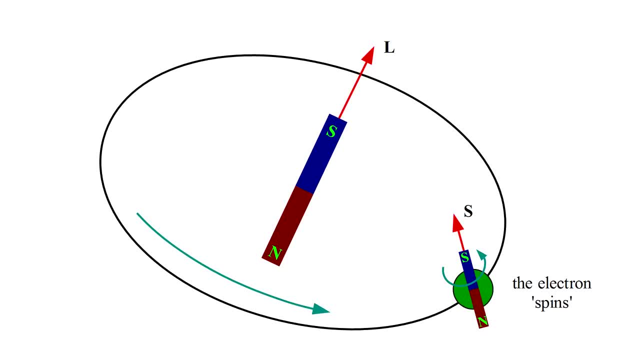 produce another little magnetic dipole. The quantum mechanical theory of angular momentum, which we briefly described at the end of video 7, tells us how a two-valuedness of angular momentum can arise. If lowercase s is the spin quantum number, then the magnitude of spin angular momentum. 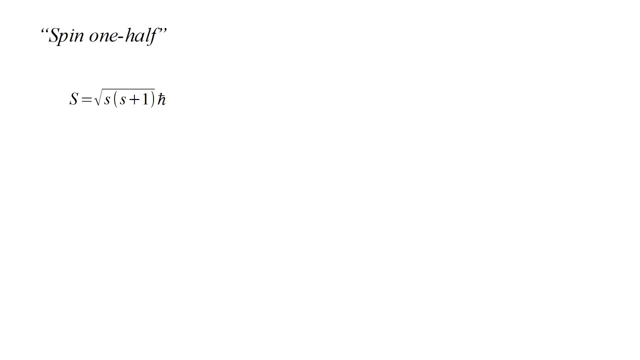 is uppercase. S equals square root of s times s plus 1 times h-bar. and recall, h-bar is Planck's constant over 2 pi. The z or up and down component is quantum number: m sub s, h-bar, M sub s takes on values minus s, minus s plus 1, up to s. 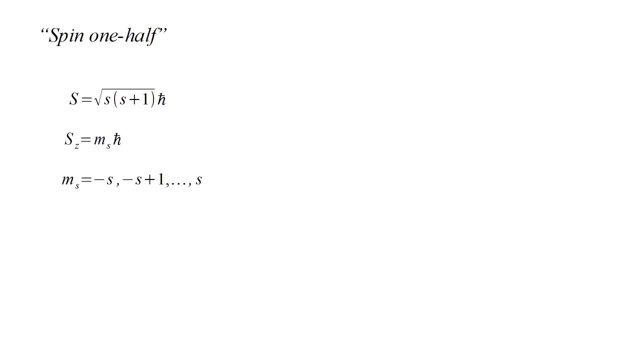 S can be zero, a positive integer or a half integer. If it's one-half, then m sub s takes on two values: minus one-half and plus one-half. A classical picture of this situation would be the electron as a spinning sphere, with 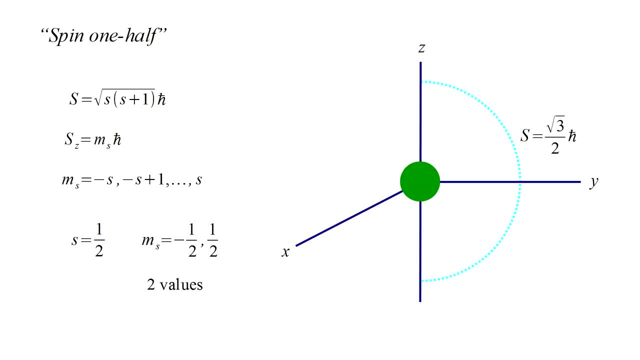 mass and charge and angular momentum of square root of 3 over 2 times h-bar. The angular momentum has a z component of minus h-bar over 2 or plus h-bar over 2, which we can refer to as spin down and spin up. 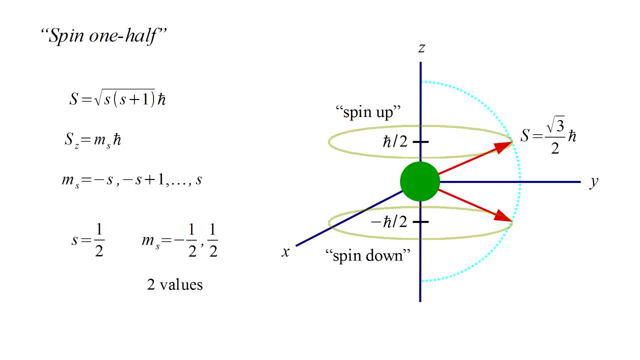 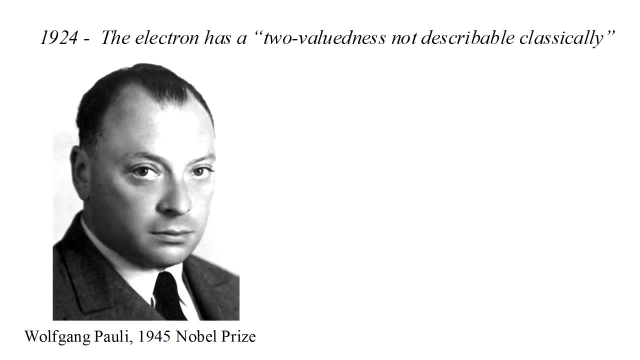 So it seems there is a classical phenomenon- the spinning of a body- that, when placed in a quantum context, can explain the two-valuedness that appears in several experiments. However, Pauli was justified in avoiding reference to classical phenomena. Let's look at an example of a phenomenon. 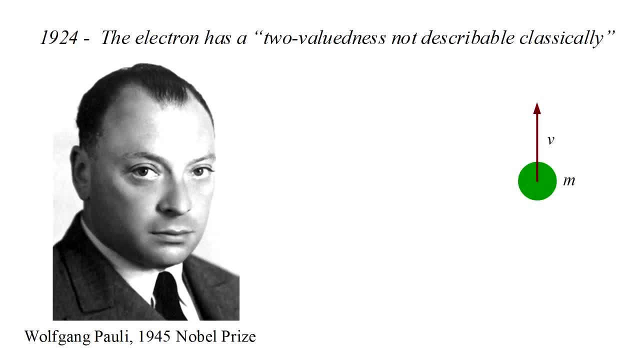 If we imagine an electron with mass m traveling with velocity V around a circle of radius r equal to the size of an atom, and we set the orbital angular momentum m V r equal to h-bar, we find a velocity that is about 1% the speed of light.